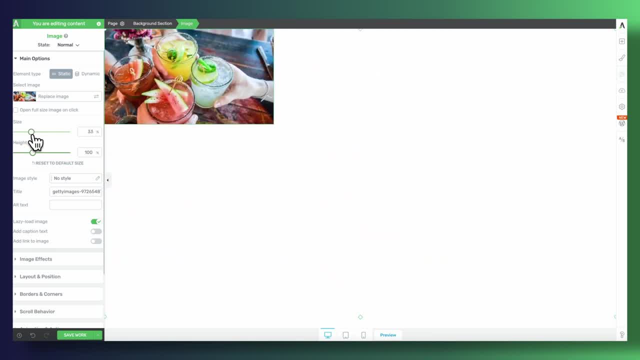 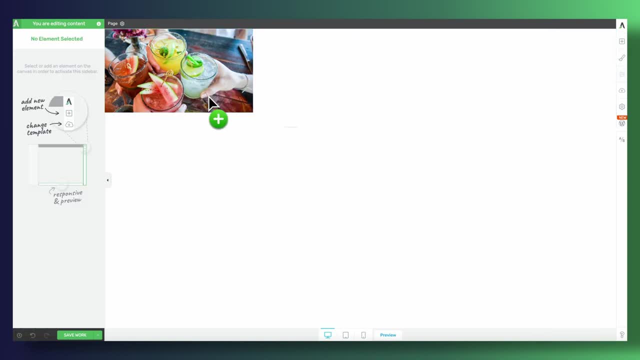 to the left-hand side of your page, towards the top or underneath the latest element that you've dropped on your canvas. And if you drop another element underneath that image, it's going to do the same exact thing. It's going to position itself underneath your image, left-aligned towards the. 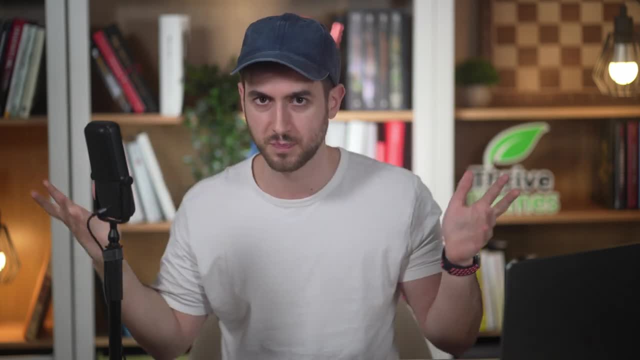 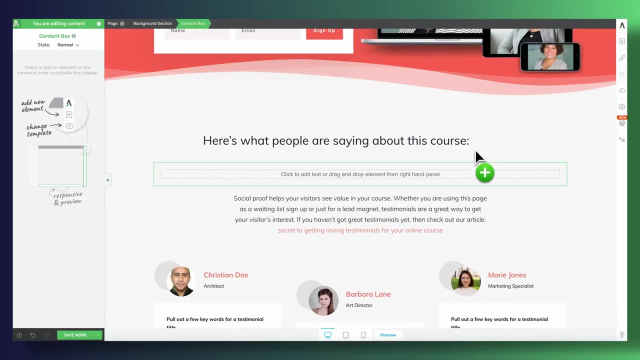 top. This is the natural flow of your page. Now, static elements can still change their position. right? You can have a text element be static, but have it sit inside a content box that is justified to the right-hand side of your page. Or perhaps you simply have your text have a maximum. 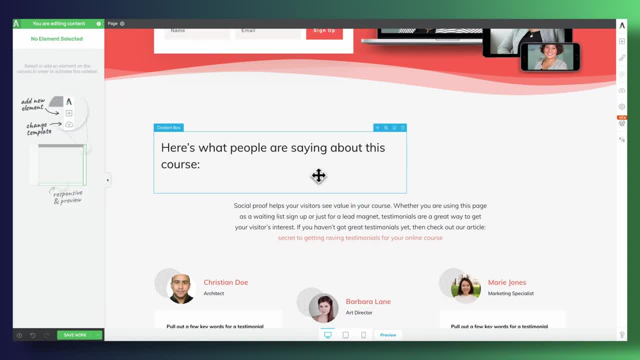 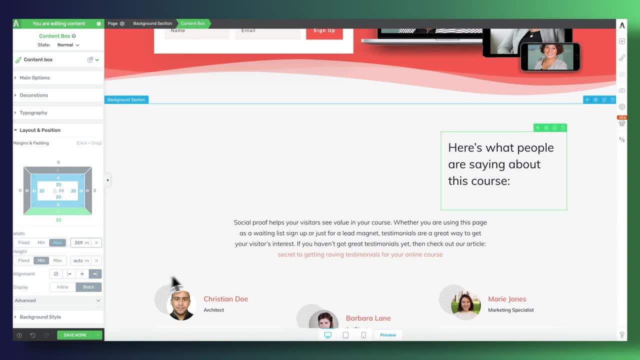 width of 400 pixels. But despite the fact that it's a static position, you can still position it to the left-hand side of your page. But despite the fact that the appearance and design of our element can change, the natural flow of our elements is to be left aligned to the top. Okay, now that we 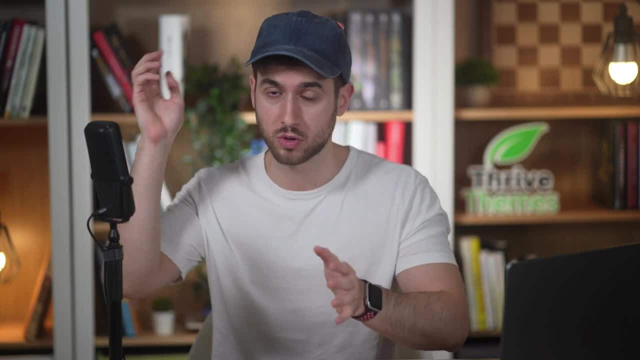 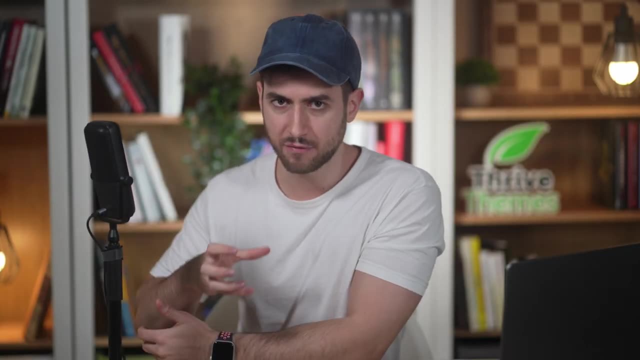 understand static positioning, and if you have any questions, you can most certainly post them in the comment section below. let's now talk about relative positioning. With relative positioning, instead of having our elements follow the default flow of our page, we're now creating a 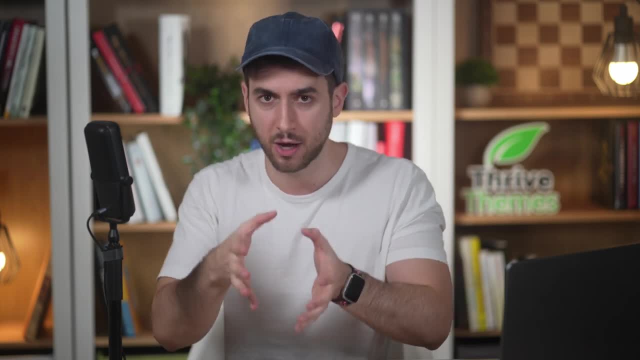 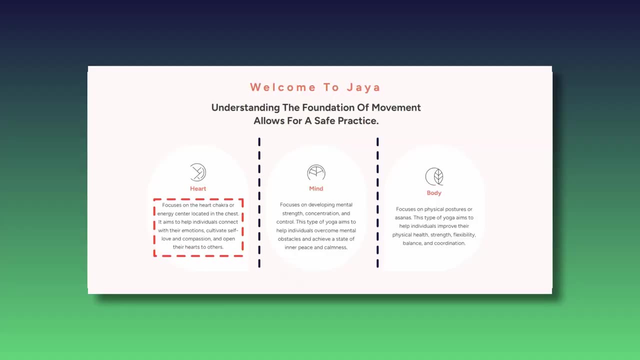 relationship between the element that we're editing and the parent container in which it sits. Let's say that we have a text element inside a column. A column would be our parent container because it holds the text element that we're editing, And so our text element would be a child. 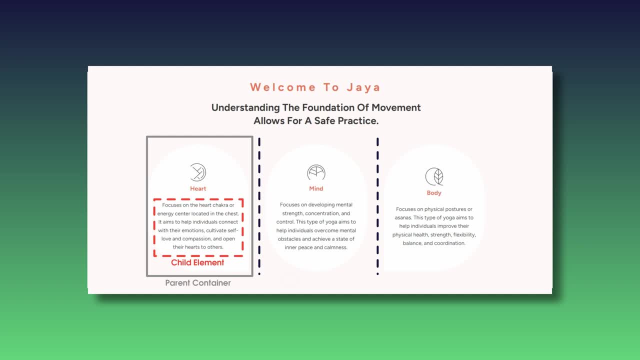 element because it has a parent container. If we set our text element to have a relative position, we're telling Thrive Architect that the position of the text element is dependent on the position of our column. Now you're going to see that by setting my text element to relative positioning. 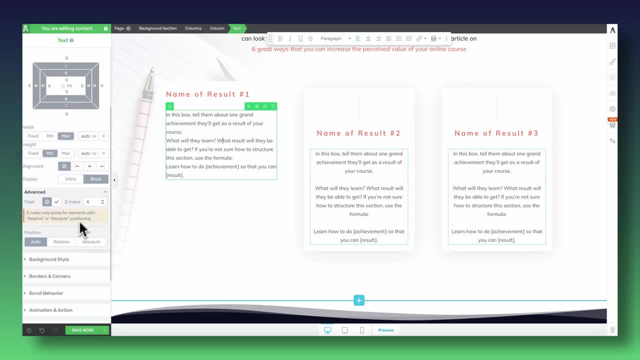 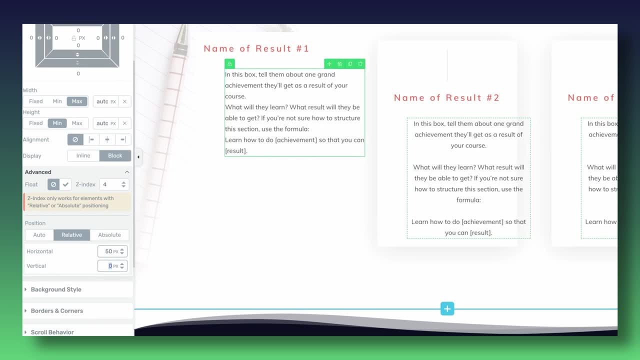 I can now adjust my vertical and horizontal values. If I were to leave these values at zero, my text element would just behave in an identical way as if it was just static. It would just follow the default flow of our page. But I can also tell Thrive Architect that I want this text element to 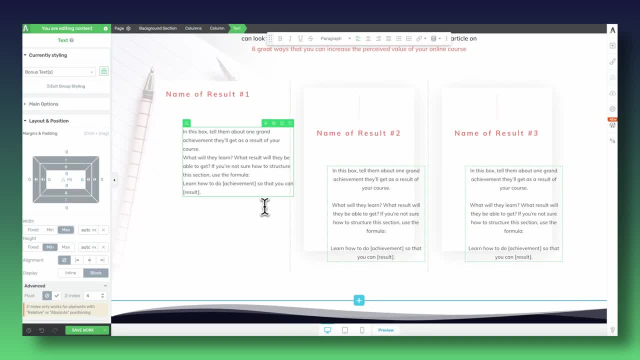 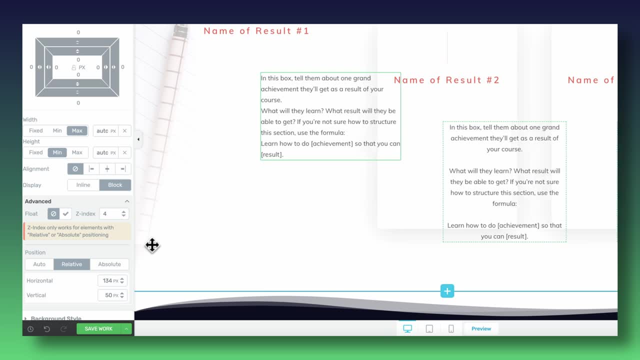 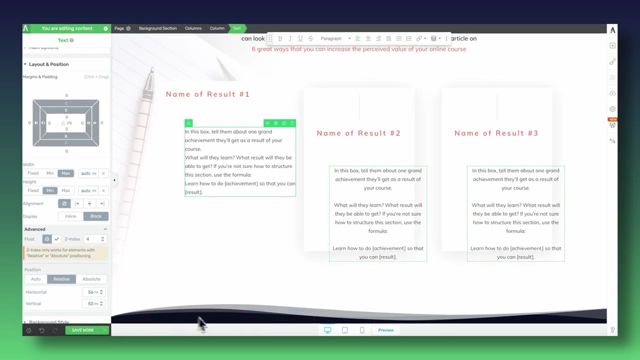 get pushed 50 pixels vertically and 50 pixels horizontally with regards to our parent container. And now, all of a sudden, by doing this, I have creative freedom to move and position my element wherever I want on my page with regards to the column in which it sits, Remember, 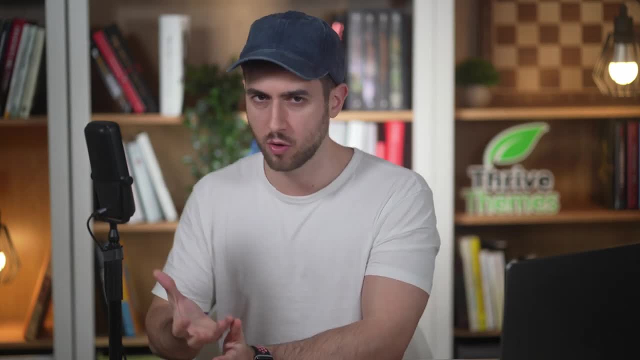 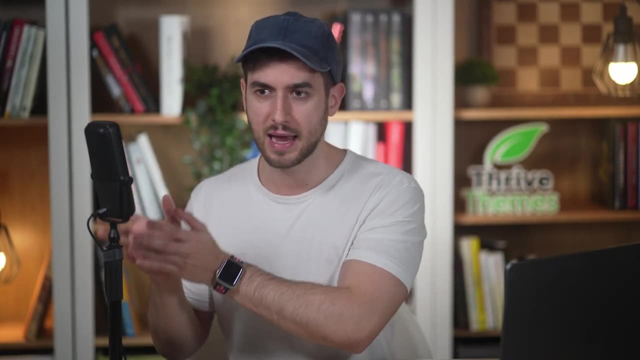 our parent container. And if you're having a hard time understanding, when would you ever do this? well, you're going to use relative positioning to create layouts on your pages where you want to have elements hanging off of the edge of other elements. Sometimes you're going to want 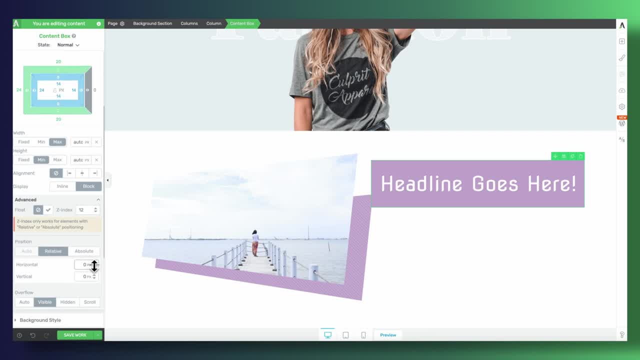 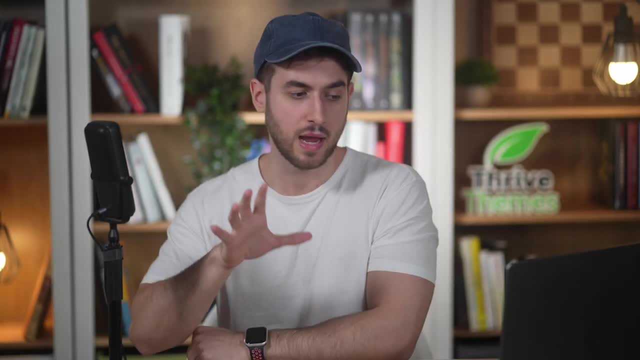 to have elements sitting on top of other elements, because breaking the natural flow of your page every now and then can lead to attractive designs, At least if you know what you're doing. I do want to answer a question that I think many of you may have, which is: 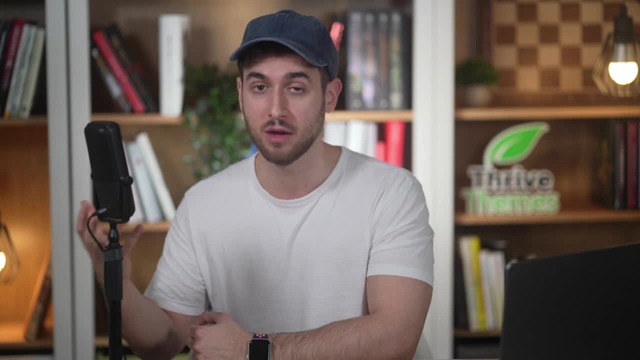 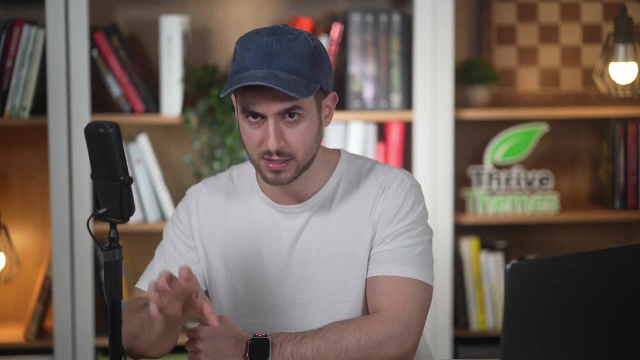 what is the difference between moving an element by having it have a relative position and moving an element by using margins or negative margins? And there's a massive difference. First of all, I truly encourage you to check out this video that I did on margins and padding if you haven't. 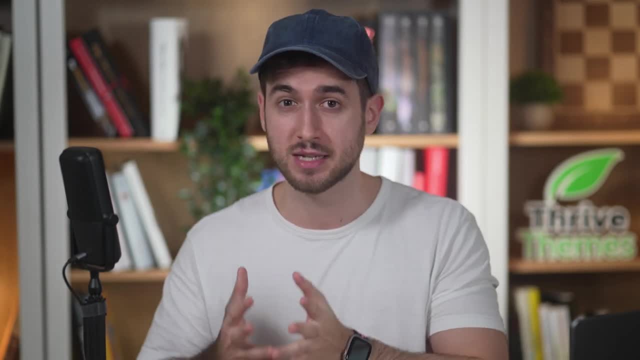 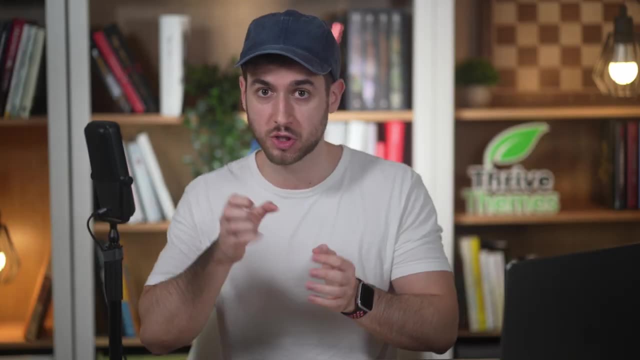 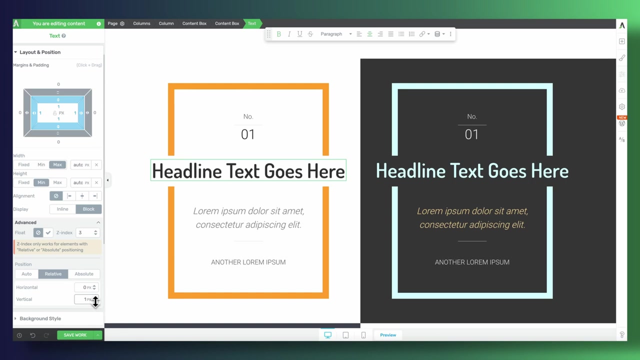 done so already. But, in summary, relative positioning doesn't affect or compromise the position of other elements on your page whatsoever, As opposed to margins which push or attract. if you're using negative margins surrounding elements, This means that with relative positioning, you can move your element wherever you want on your page. It's. 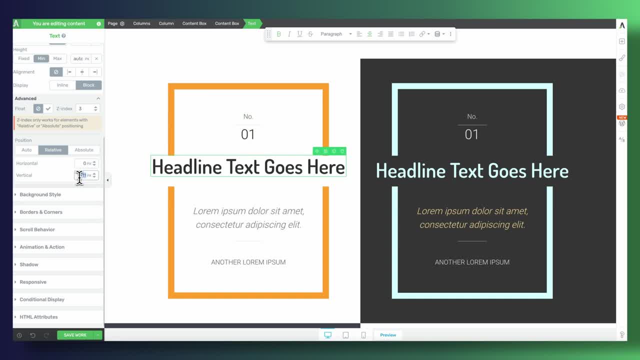 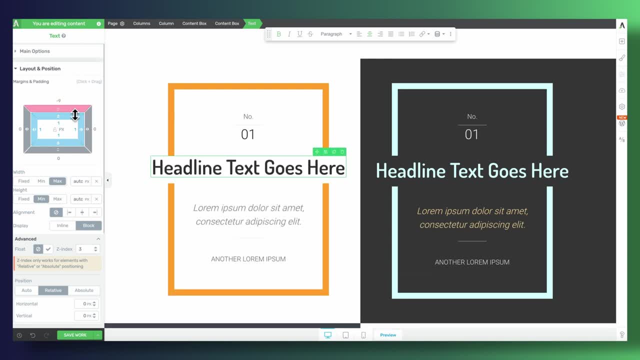 not going to impact the placement of other elements whatsoever, But when you're using margins, you will see that whether you're using positive or negative margins, you're going to be pushing or bringing with you other elements as well. Okay, now let's quickly talk about absolute. 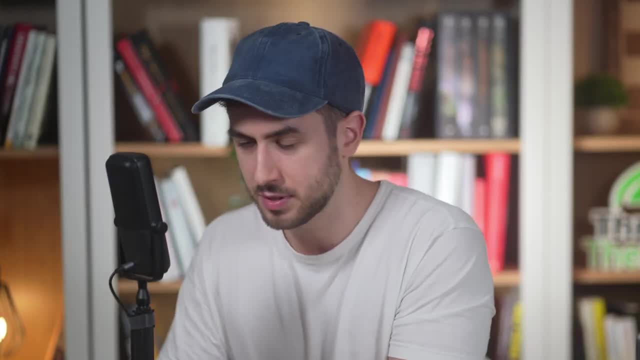 positioning. I think this one's a little bit easier to understand. Absolute positioning works in a similar way when you're using positive or negative margins. If you're using positive or negative margins, you're going to be pushing or bringing with you other elements as well. So 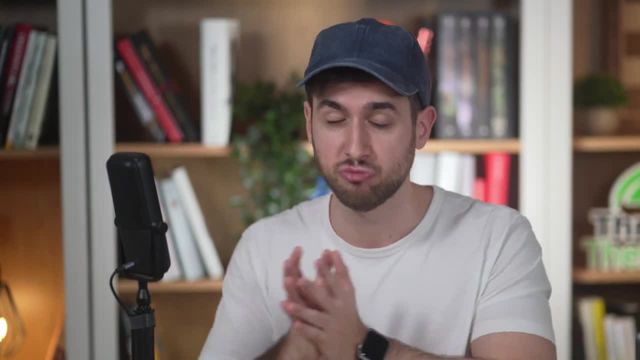 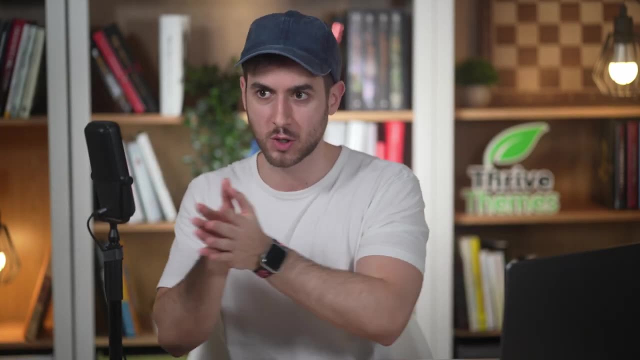 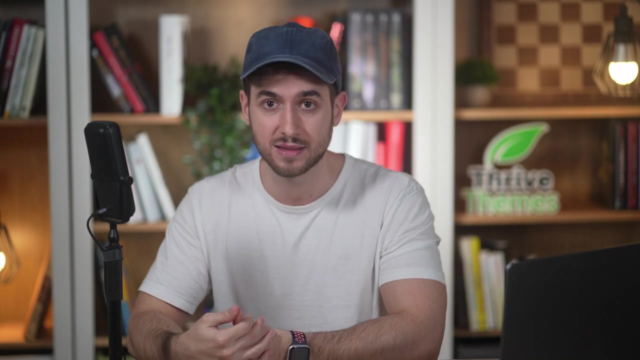 relative positioning works in a similar way to relative positioning, in the sense that we are creating a relationship between a child element and a parent container, But instead of having our element move horizontally or vertically, we're having it sit in a fixed location, And if you're using Thrive Architect, you'll quickly see that these locations can be. 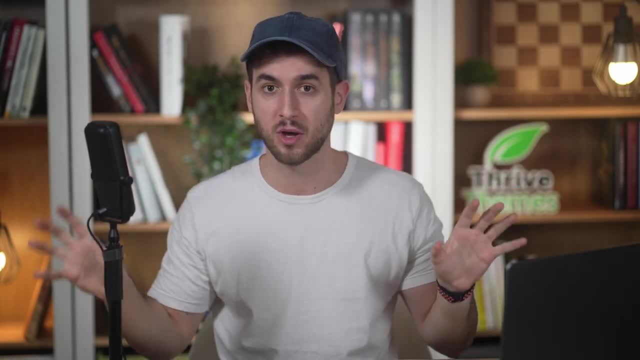 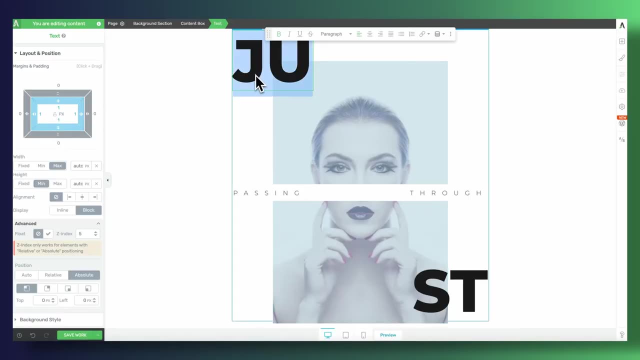 either the top left, top right, bottom left or bottom right corners of our parent container. Let me just give you a quick example. If you have a content box, you can have an image at the top left corner of that content box or at the bottom right corner of that content box.